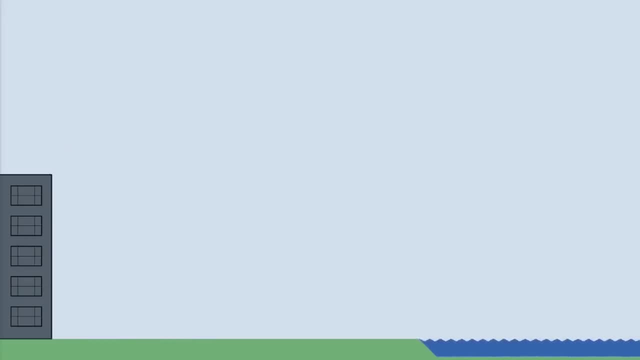 higher is not enough to compensate for the loss of horizontal velocity. So you go home and you sit at your desk, define some variables, draw some diagrams, work out the formula for the time spent in the air, Multiply that by the constant horizontal velocity to get the distance, and then you find the maximum. 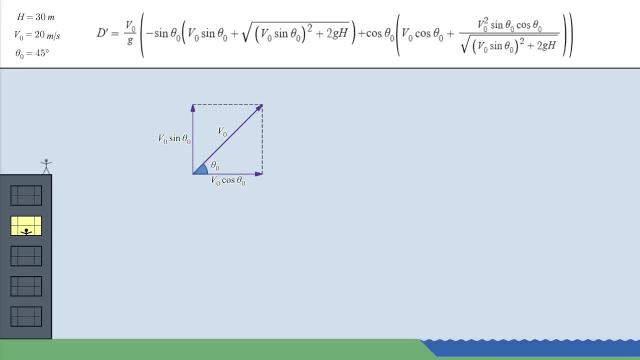 of that function by simply taking its derivative, setting it to zero and solving for the launch angle. And then you realize that that last step is impossible and you've reached a dead end. Well, if you're like me, it's happened at least once, And in that case, this video is for you. 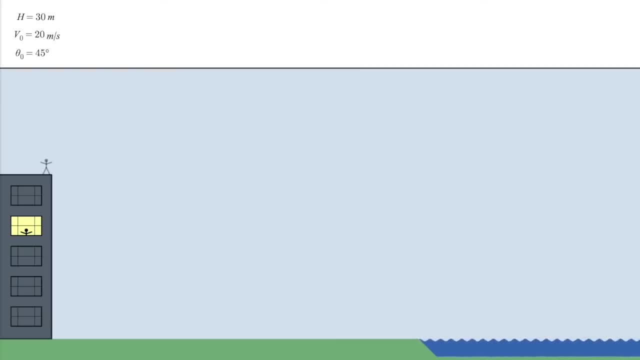 To figure this one out, we need a change of perspective. Instead of tracking the direction of the projectile, let's take a close look at its velocity. We can represent velocities with rays which point in the direction of motion and whose length represents how fast it's moving. 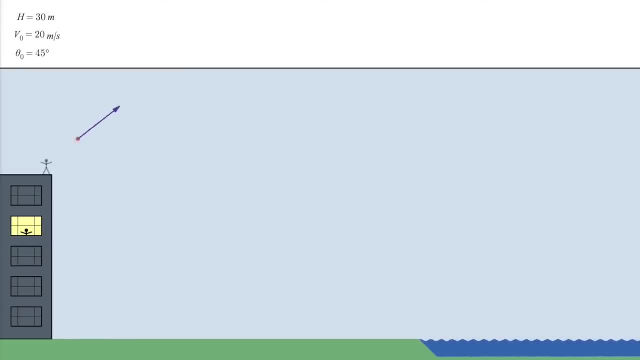 At the start, the ray will look like this And as it travels along with the projectile's parabolic path, it changes continuously due to gravity, until it hits the ground at a larger speed and a downward angle. To be clear, I'm assuming ideal conditions, ignoring air resistance. 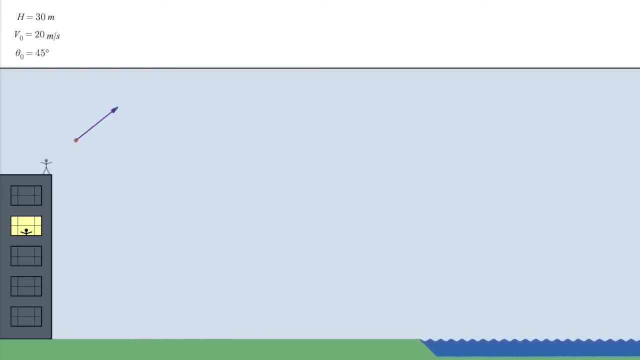 assuming the curvature of the earth is negligible and sticking to Newtonian physics. Also, I'm assuming that you can throw with the same speed at any angle, which probably isn't quite true. Keeping all that in mind, we can solve this problem without too much difficulty. First, it's useful to think of the velocity at any point, as 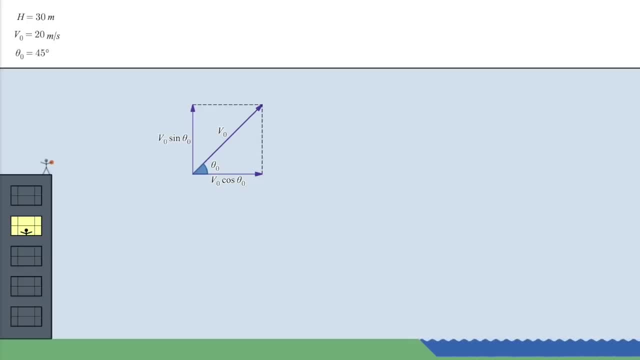 the sum of a horizontal vector and a vertical vector, since the vertical component determines how high the projectile will be at any point in time and the horizontal component tells us the rate at which the projectile is moving away from the middle. So if you're going to do this, you 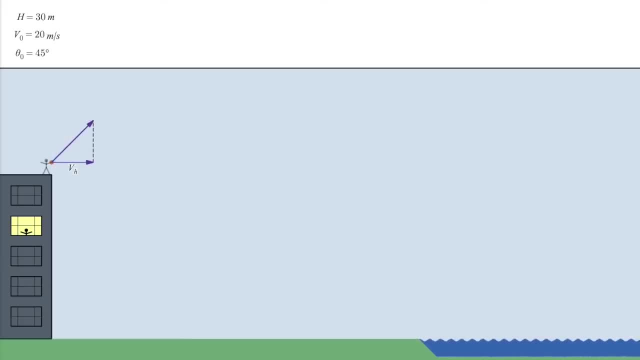 can use the horizontal vector to calculate the velocity at any point in time. Notice that the horizontal component doesn't change throughout the flight. Since gravity acts only in the vertical direction, it can change only the vertical component. And since gravity is the only thing changing the velocity, in this ideal scenario nothing will change. 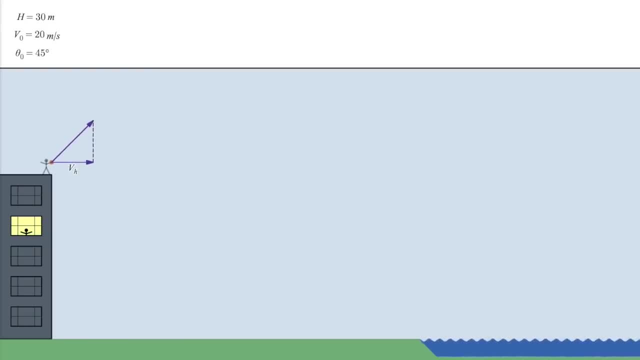 that horizontal speed. This means that the final distance can be computed by multiplying the total airtime by the horizontal velocity. Now let's look closely at how the overall velocity changes during the flight. If we bring all these rays together, we can see more clearly how the velocity changes. 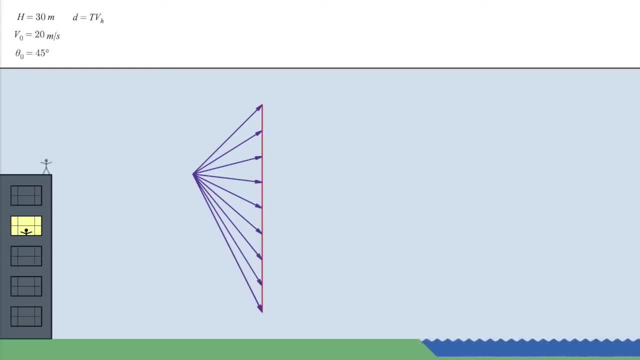 Notice that the line connecting the ends of these rays is vertical. Why? Because this line represents the total change in velocity and, again, the only thing changing the velocity is gravity. And since gravity is constant, we can quantify this change as the gravity of Earth about. 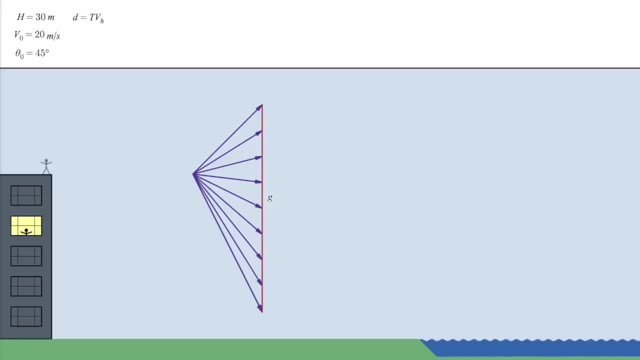 7.8 meters per second squared, multiplied by the total airtime. whatever that may be, Let's look just at this triangle. The upper side represents the velocity of the throw and the lower side represents the velocity when the projectile hits the ground. 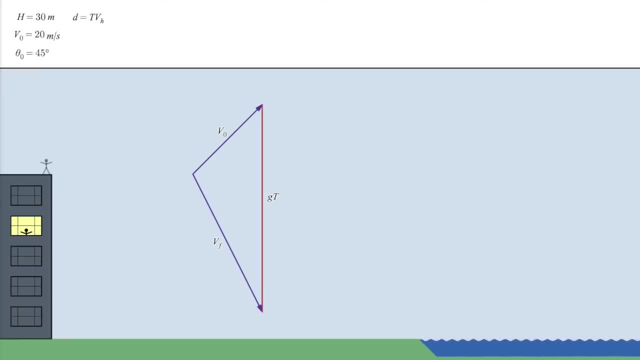 Interestingly, its speed when it hits the ground doesn't depend on the angle of the throw. That's because of the conservation of energy. The energy of motion, kinetic energy, when the object reaches the ground must be equal to the kinetic energy, The energy of the throw plus the potential energy that comes from the starting height. 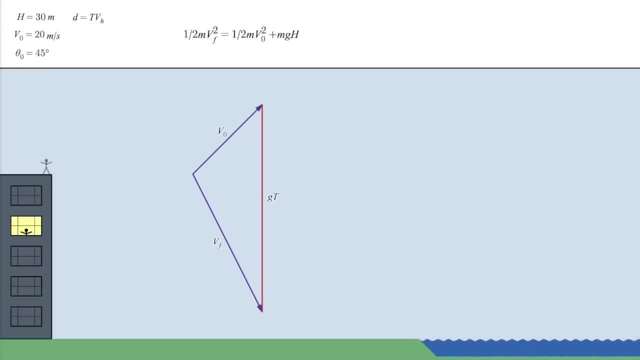 Well, at least in our idealized scenario where no energy is lost to air resistance. So for the purposes of finding the best launch angle, we can treat the magnitudes of the initial velocity and the final velocity as constants. We know a lot about this velocity triangle, but what does it have to do with maximizing? 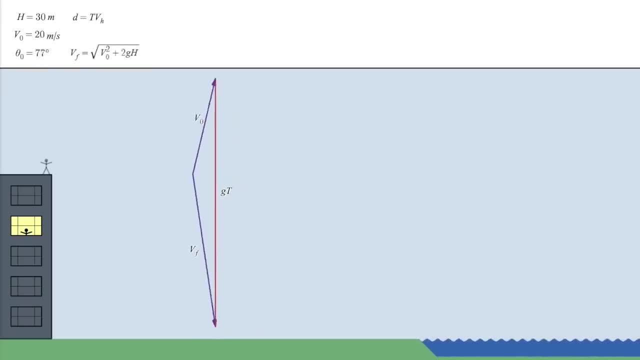 the distance. Well, you might notice that when the throw goes straight up, so that the total distance is zero, the triangle flattens into a line, And it's the same when the throw goes straight down. This might make you wonder if the distance is somehow related to the area of the triangle. 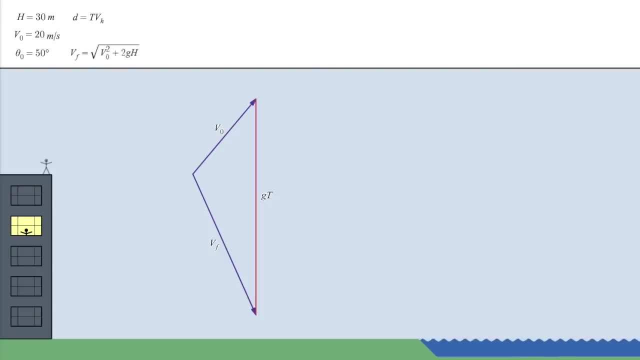 Well, check this out. The area of the triangle is one half the base which we can take to be this line times the height which would be this line which, as we've already seen, represents the horizontal velocity. So the area of the triangle is one half gt times vt. 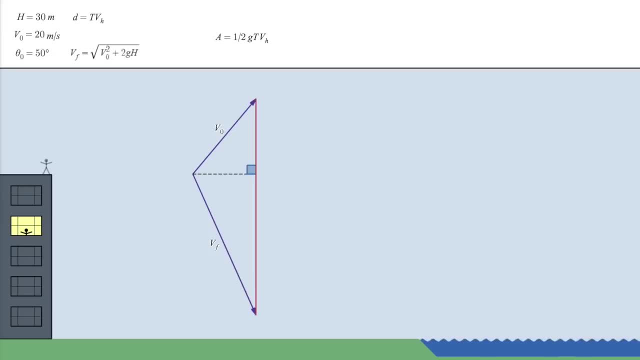 So that's one half. This is vh, which differs from the distance by a factor of one half, g, which is a constant. In other words, if we find the launch angle that maximizes the area of the triangle, we'll have the angle that maximizes the distance. 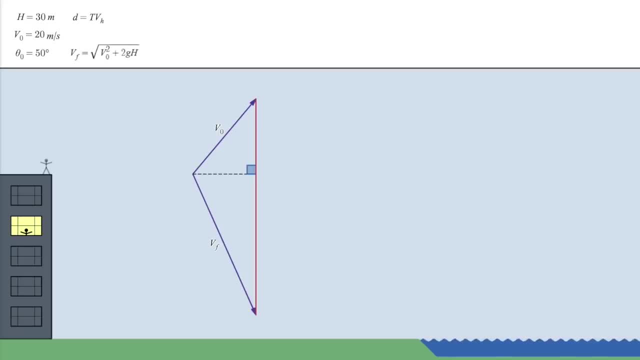 So when is the triangle's area maximized? Well, if we now choose the final velocity as the base, then, since that's a constant, we just need to find the angle that maximizes the height, which is this line here. Notice that this line is always shorter than the initial velocity line, except when they're